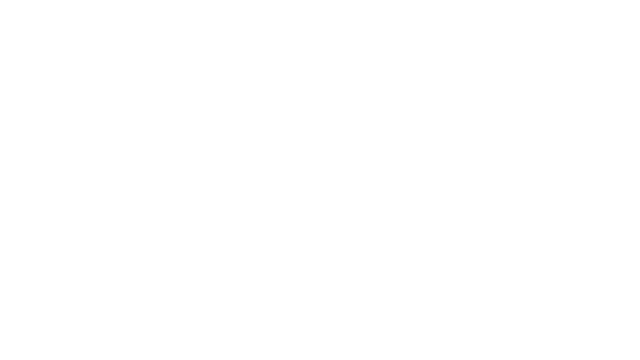 need any experience or knowledge to learn programming whatsoever, So you can be a complete novice and not know any sort of code or anything about computers. that doesn't matter In this case. you guys can learn for free and easily. The second thing is you don't need to pay. 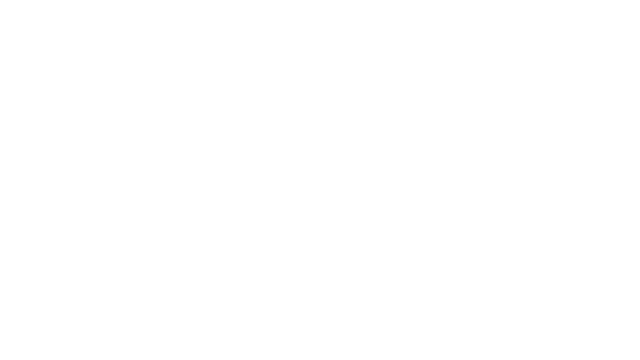 a single cent for this and it will always be free. There are those services where you sit down on the computer and you're learning something and then you notice like a week later the trial ended and then you have to pay. That's not going to happen Again. this. 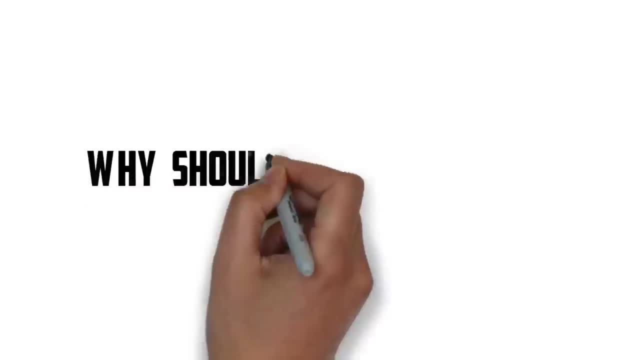 is completely free, so you don't have to worry about that. So, with that being said, why should you learn to code or to program? It's simple: When you guys learn programming, you can be comfortable with it. You can learn to code, you can learn to program. you can learn to. 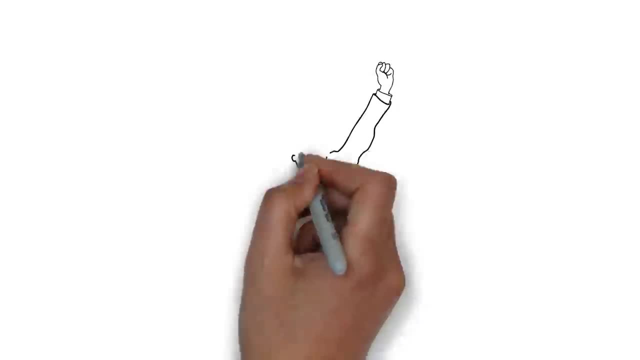 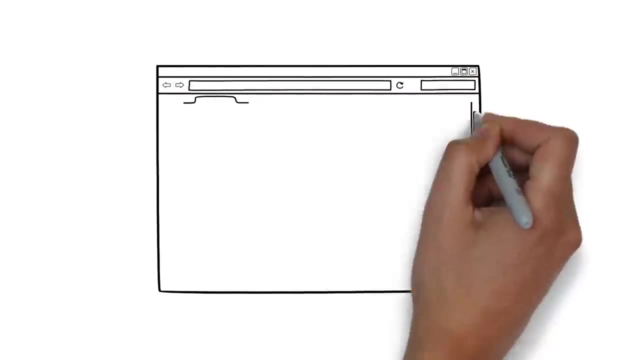 program, a web developer and later on, a full stack developer. So you can be sitting at home on a computer drinking your coffee learning the code. and then, a couple months later, you go on the online web and you go to freelancing sites and like upworkcom and 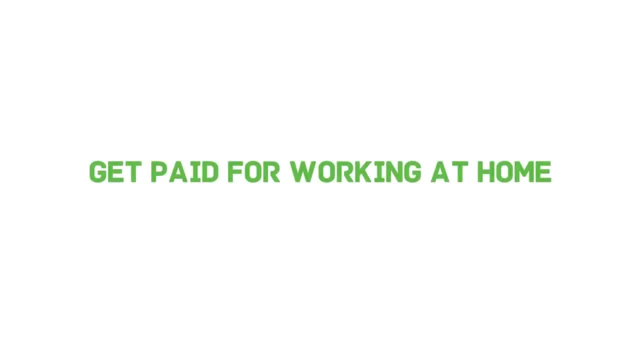 then you start making money and you help people out and you get paid for working at home. I know countless of people my age and younger than me that are 16 making hundreds and even thousands of dollars a month. So it's all worth it. How do you get started? I'm going. 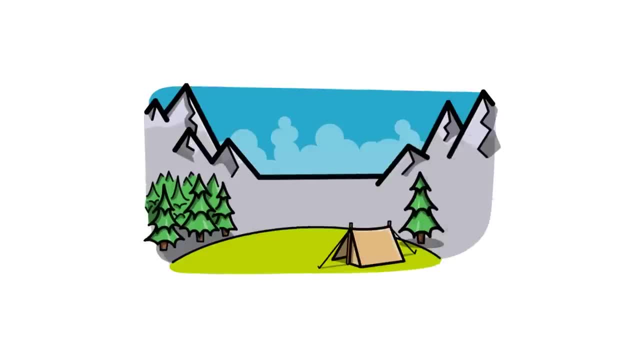 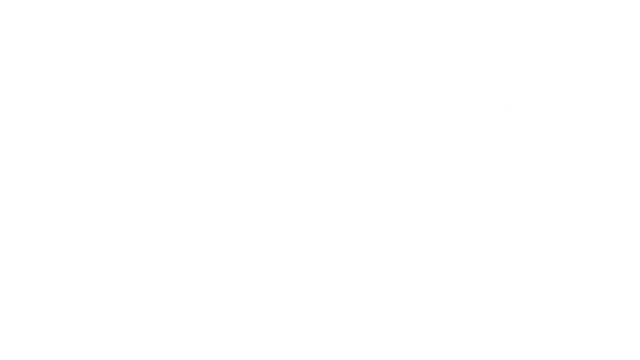 to show you guys that right now It's a free website that you guys can see down in the description link below, called freecodecamporg. Now I'm going to go ahead and show you guys this, but real quick, just so you guys know, as a disclaimer, I do not own the site and I am not affiliated with. 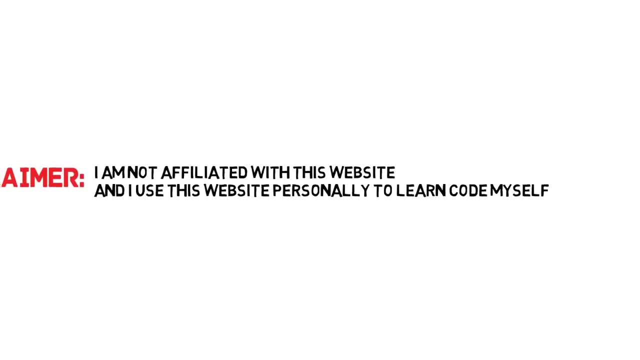 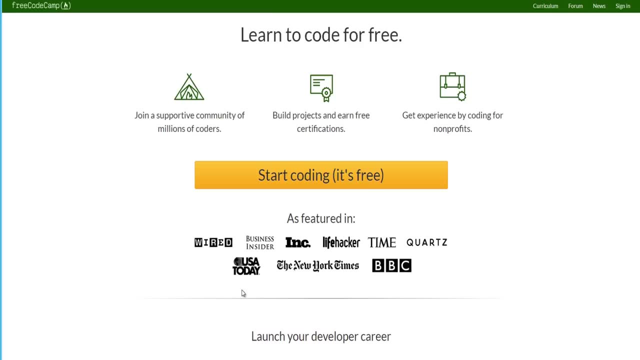 the site. I personally use this website to learn code myself, which is why I'm spreading the word and spreading the knowledge to you guys. So, with that being said, let's begin. Okay, so we're here at freecodecamporg Now to start. it's simple. All you guys got to do is 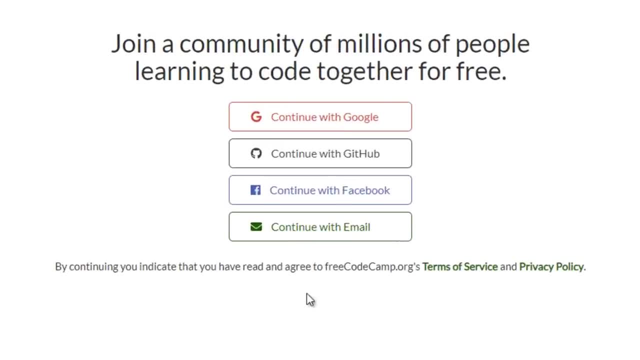 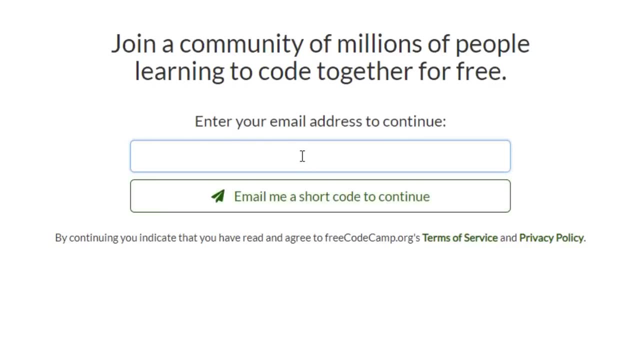 click the orange start coding button right here, And from there you guys can go ahead and continue with Google or with Facebook or with email, It doesn't matter. I'm going to go ahead and, just for this example, put in the temp email, just to show you, guys, you 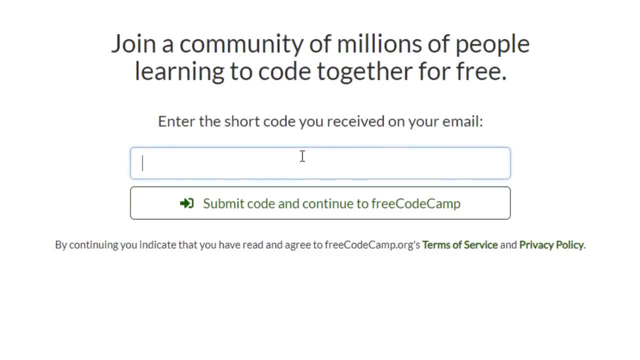 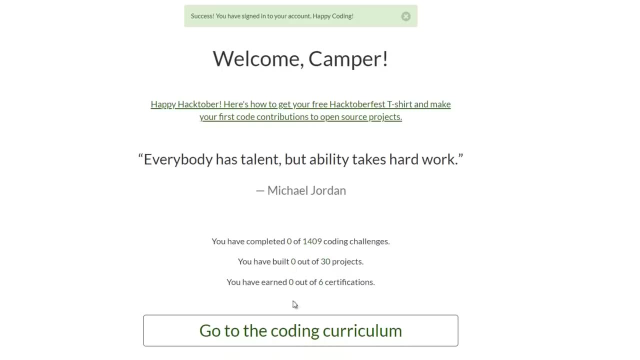 can do the same thing. Put in an email address, email and then put the code in that you get from the email and then click submit code and continue the free code camp And from there all you guys are going to do is click on the go to coding curriculum Once you guys. 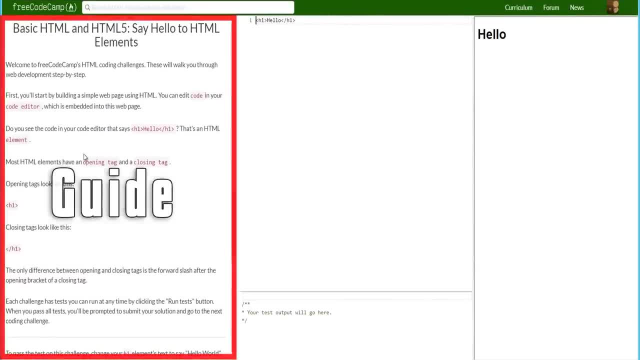 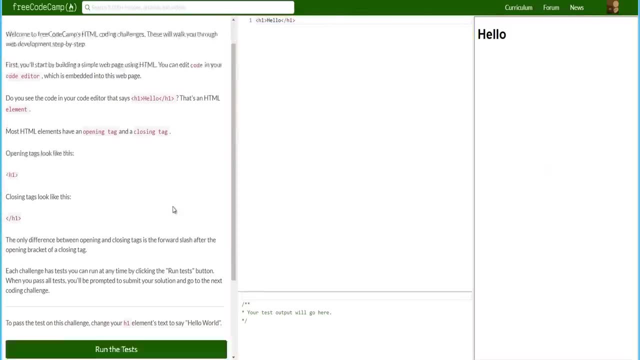 are on a coding curriculum. you're going to get three sections of the screen: The guide section, the editor section on the center and the live production section on the right side of the screen. So, following the left side of the screen, you guys are going to get a. 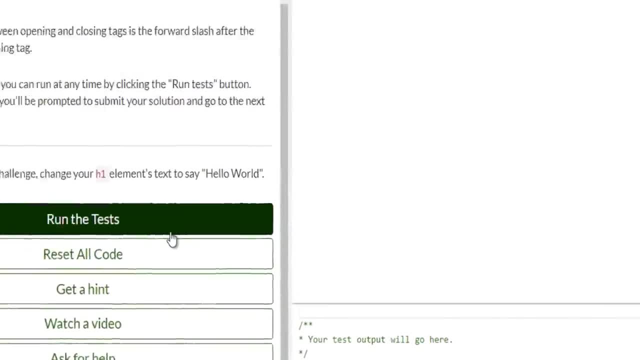 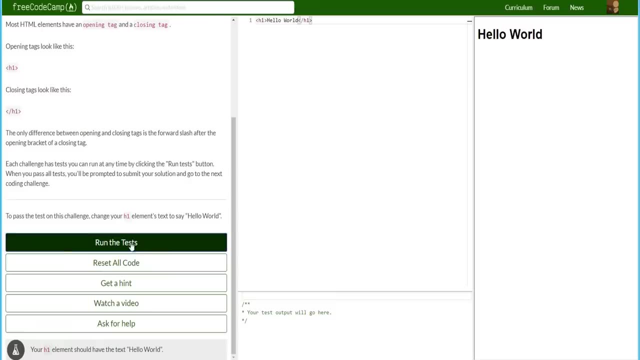 tutorial and then you're going to get a little challenge. You guys are going to have to pass the challenge. So in this case, I'm going to go ahead and have to do an H1 element and type in: hello world. That's what it's asking you to do. Run the test. You can see we did it And then we 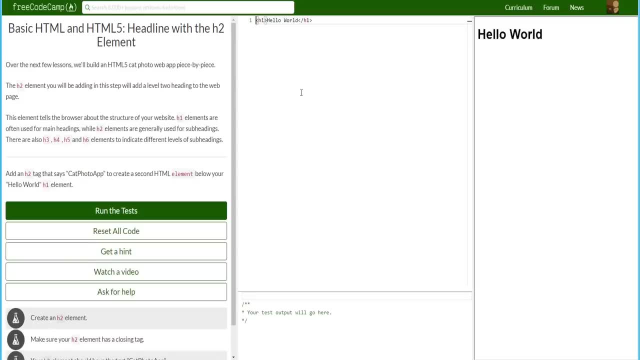 go to the next challenge. The next challenge again. you just got to follow the instructions. So an H2 element and do a cat photo app text. So do that And you guys get the idea. Basically, what you guys want to do is make sure you follow the instructions carefully. I highly recommend you. 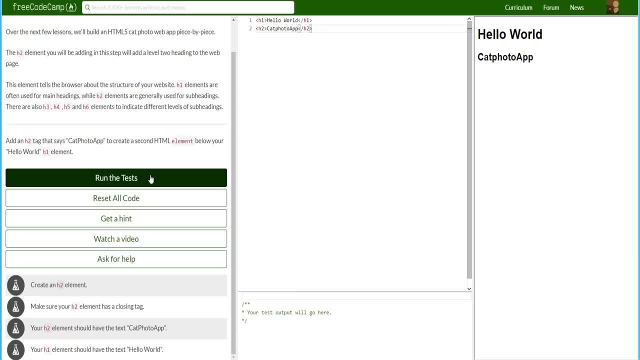 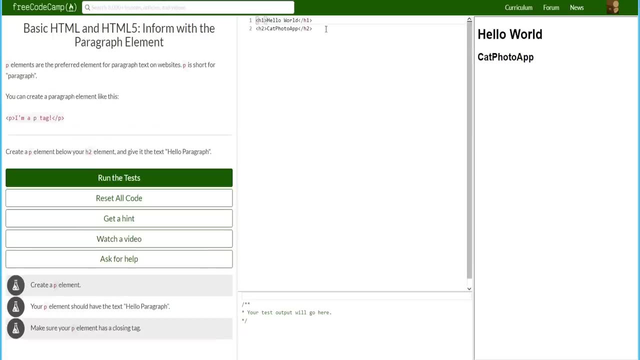 guys get a notebook and take notes along the way. It does get very easy. It is very easy to start with, but it will get more and more challenging And if you guys are getting stuck while doing this, you don't have to worry. You can click on, get a hint and it'll give you guys a hint on what to do. 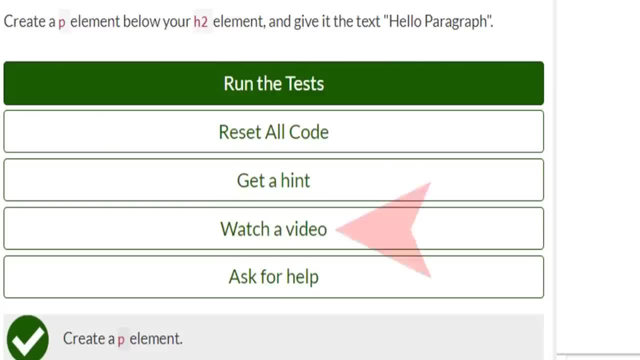 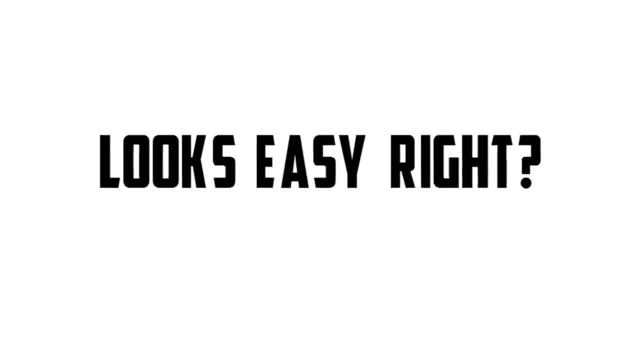 And you want to see how you can do it, how you can pass it, Then you can watch a video and it'll tell you exactly what you did wrong and show you the right way. And that's pretty much it. So, in conclusion, we learned that there's a program you guys can use and it does look simple. 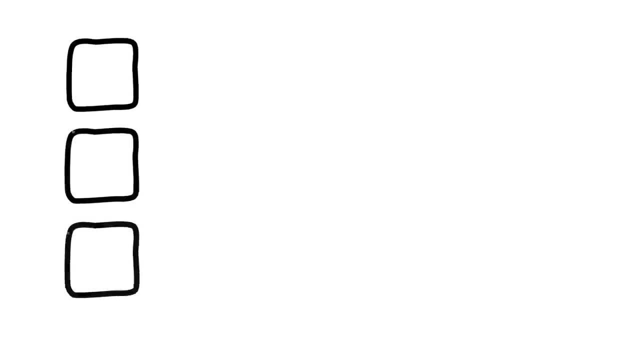 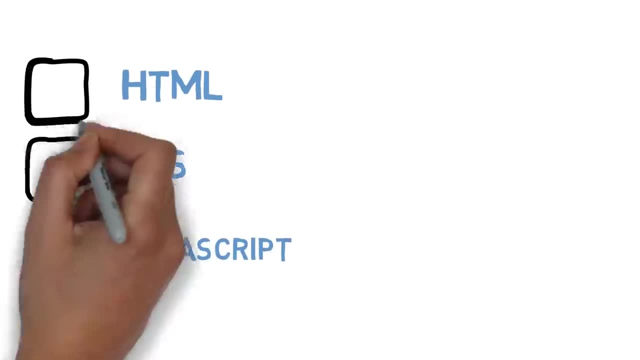 at first, but it progresses and gets more difficult. So you guys are responsible for sitting through the lessons and trying to check off each of the lessons you guys learned, beginning with HTML, and then CSS, visual design and eventually JavaScript. There's hundreds and 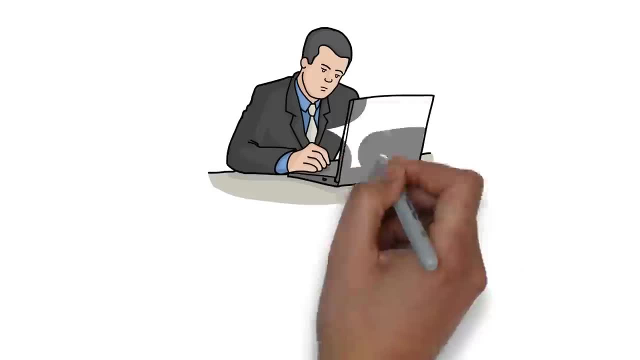 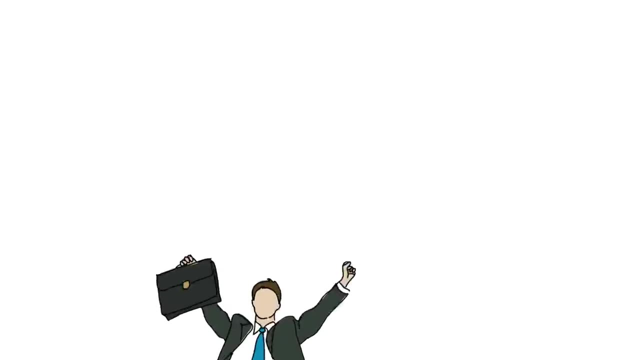 hundreds of, countless of hours of free learning you guys can get with this. You're going to be sitting there and thinking about the challenge. You're going to be like, wow, this is very difficult. How do I move on to the next challenge? So you really have to test yourself and take notes. As I mentioned, it will really